So that's v. That's v plus w. It's negative i plus 2j. 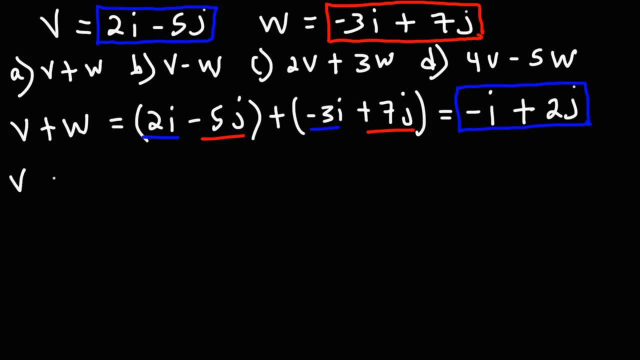 Now let's move on to part b. So what's v minus w? 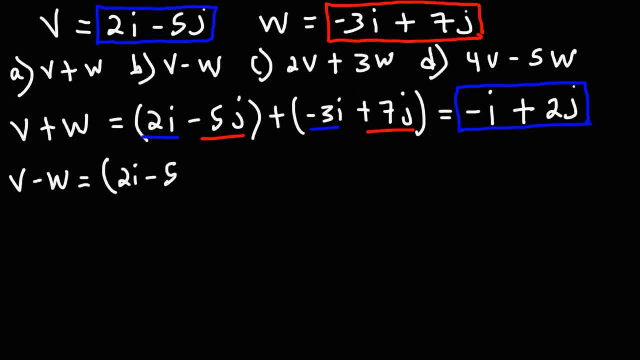 So this is going to be v, 2i minus 5j. 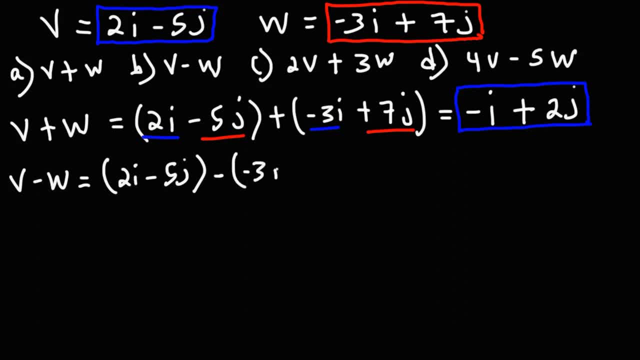 And then minus w, which is negative 3i plus 7j. 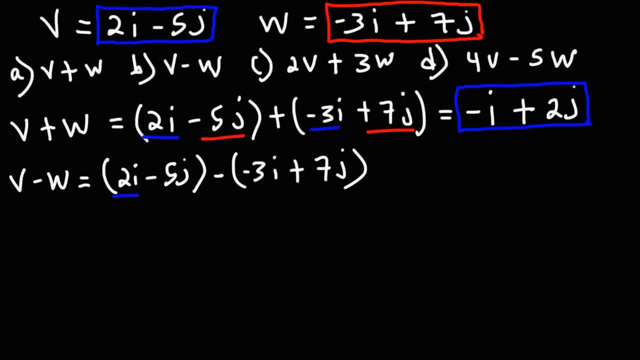 So 2i. Well, let's rewrite it first. Let's distribute the negative sign. So this is 2i minus 5j. And then negative times negative 3i. So that becomes positive 3i. And then negative times 7j. That becomes negative 7j. 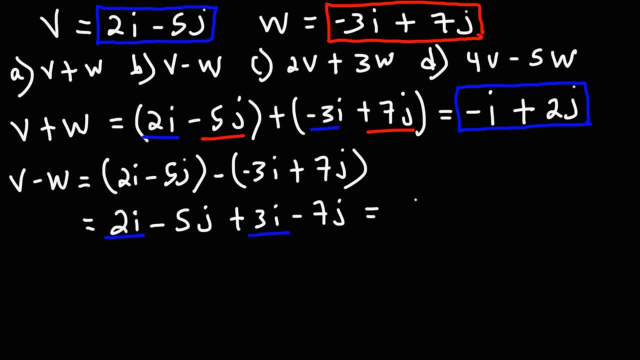 So now let's combine like terms. 2i plus 3i is 5i. And negative 5j plus negative 7j. And then negative 5j. And that's going to be negative 12j. 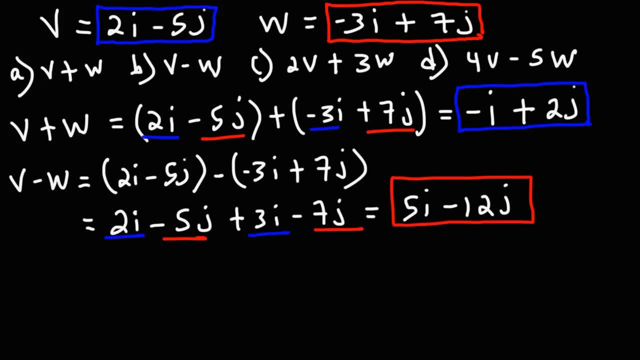 So that's v minus w. So we get 5i minus 12j. 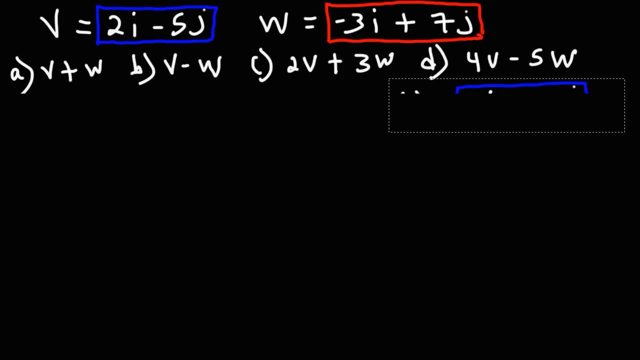 Now let's clear what we have to make some space. Now let's move on to part c. 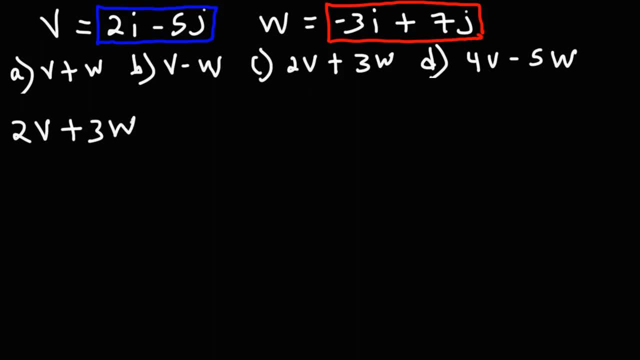 So we have 2v plus 3w. So now, not only are we adding vectors, we're also multiplying these vectors by scalar quantities. We're multiplying vector v by the scalar quantity of 2, and we're multiplying vector w by the scalar quantity of 3. 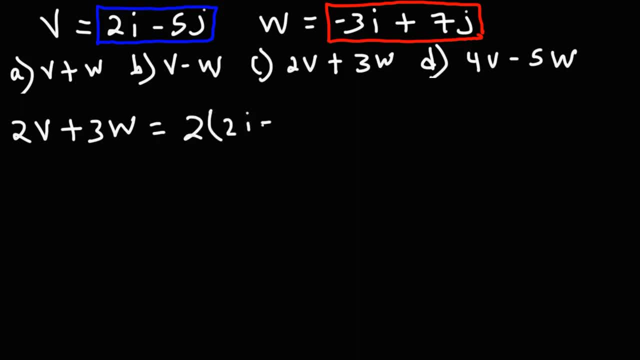 So we have 2v, so 2 times 2i minus 5j, and then plus 3w, or 3 times negative 3i plus 7j. So let's begin by distributing. 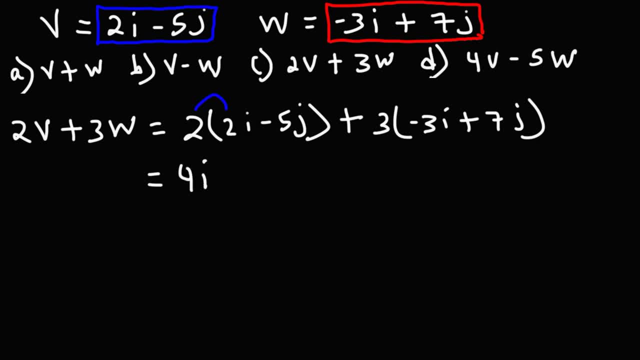 So 2 times 2i is going to be 4i. And then 2 times negative 5j, that's negative 10j. And then we have 3 times negative 3i, that's negative 9i. And then 3 times 7j, that's 21j. So now let's combine like terms. Let's combine like terms. 4i minus 9i is going to be negative 7j. Negative 5i. 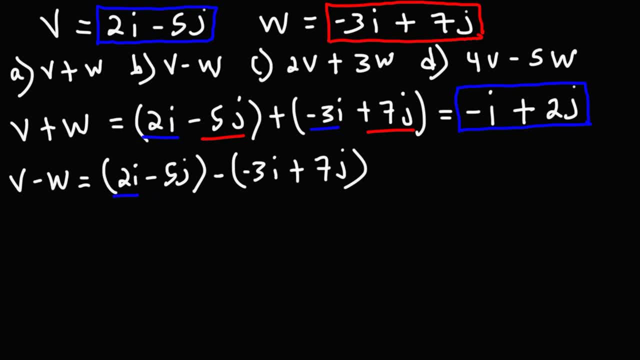 So 2i. Well, let's rewrite it first. Let's distribute the negative sign, So this is 2i minus 5j, And then negative times, negative 3i, So that becomes positive 3i, And then negative times 7j. 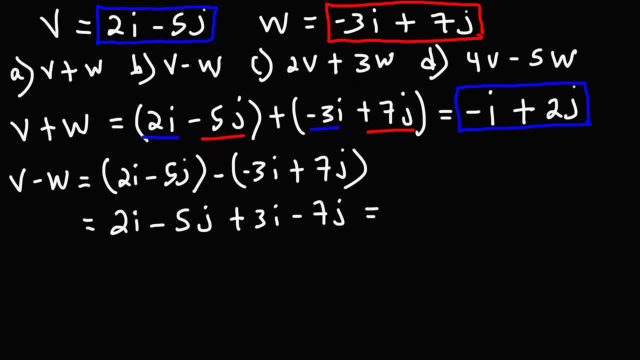 That becomes negative 7j. So now let's combine like terms: 2i plus 3i is 5i And negative 5j plus negative 7j And then negative 5j. That's going to be negative 12j. 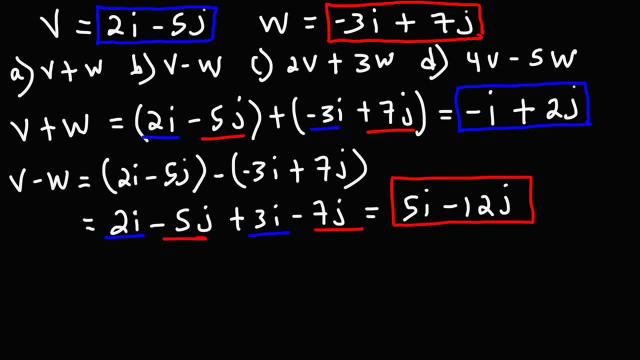 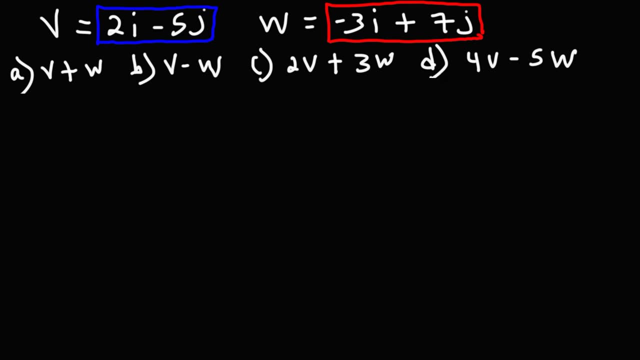 So that's v minus w. So we get 5i minus 12j. Now let's clear what we have to make some space. Now let's move on to part c. So we have 2v plus 3w. So now, 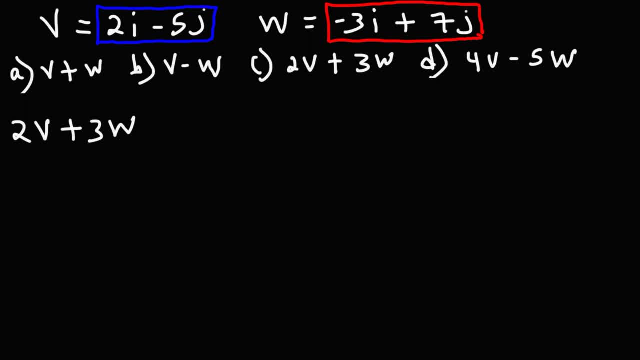 not only are we adding vectors, we're also multiplying these vectors by scalar quantities. We're multiplying vector v by the scalar quantity of 2.. And we're multiplying vector w by the scalar quantity of 3.. So we have 2v. 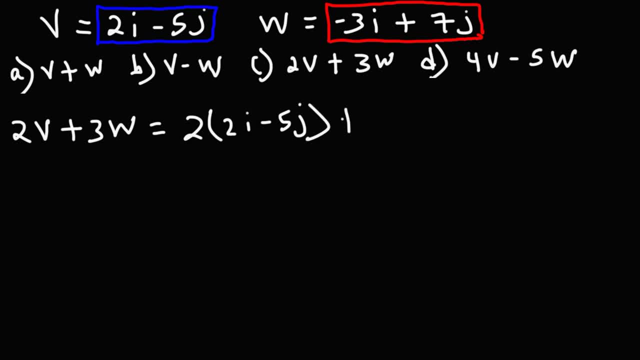 So 2 times 2i minus 5j, And then plus 3w, or 3 times negative 3i plus 7j. So let's begin by distributing. So 2 times 2i is going to be 4i. 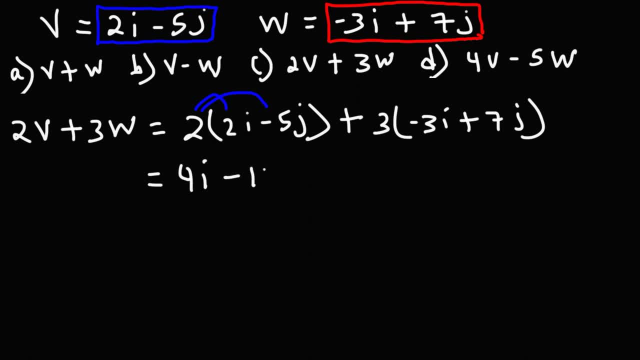 And then 2 times negative 5j, That's negative 10j. And then we have 3 times negative 3i, That's negative 9i. And then 3 times 7j, That's 21j. 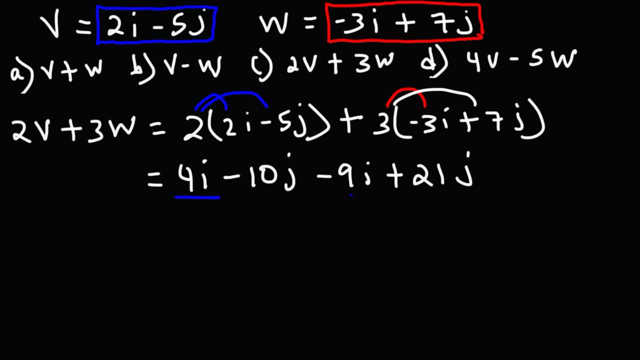 So now let's combine like terms: 4i minus 9i is going to be 9j. 4i minus 9i is going to be 9j. 4i minus 9i is going to be 9j. 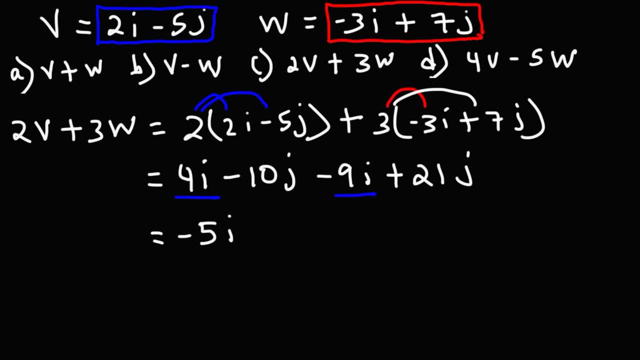 going to be negative 5i, and then negative 10j plus 21j, So that's going to be positive 11j. So that's it for the first problem. I mean problem number C. Our final answer is negative 5i plus 11j. 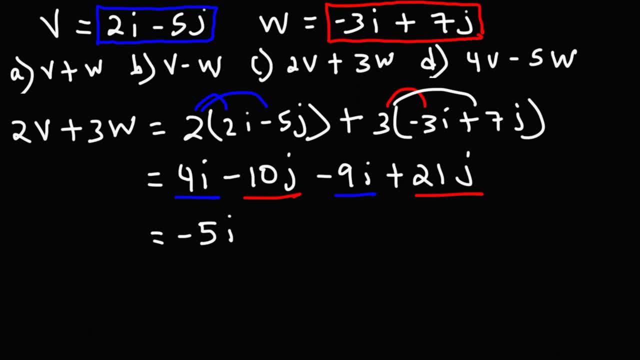 And then negative 10j plus 21j. So that's going to be positive 11j. So that's it for the first problem. I mean, problem number c. 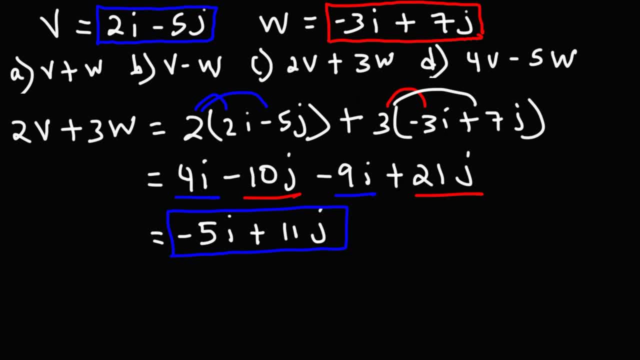 Our final answer is negative 5i plus 11j. 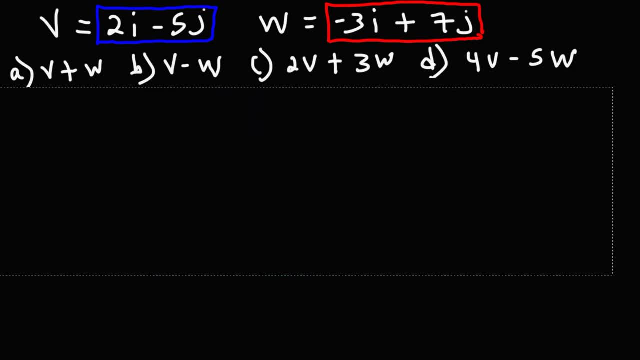 Now, feel free to pause the video and try part D if you want to. 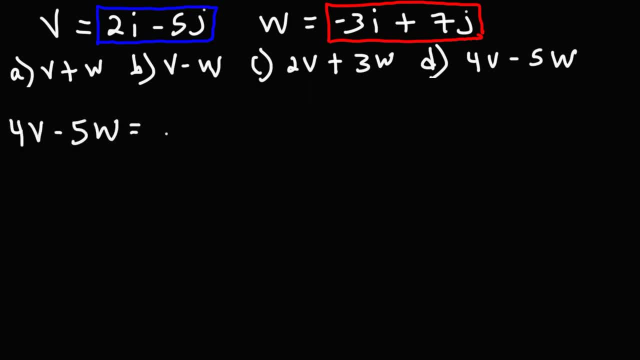 So we have 4v minus 5w. v is 2i minus 5j, and then minus 5 times w. So just like before, we're going to distribute. 4. Times 2i is 8i. 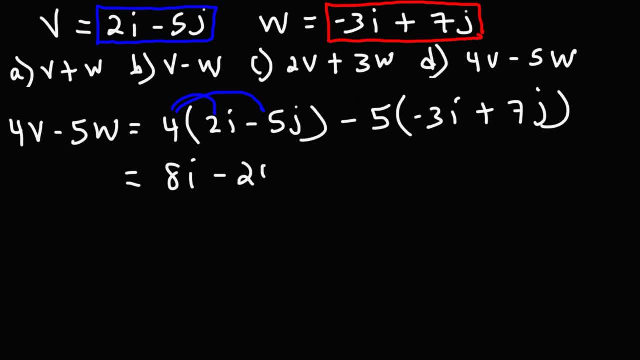 And then 4 times negative 5i is negative 20. 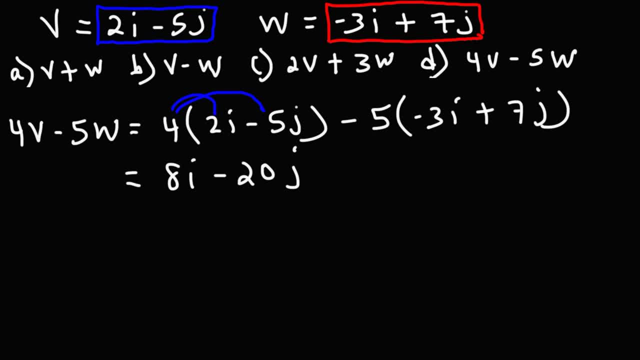 I meant to say 4 times negative 5j. That's negative 20j. 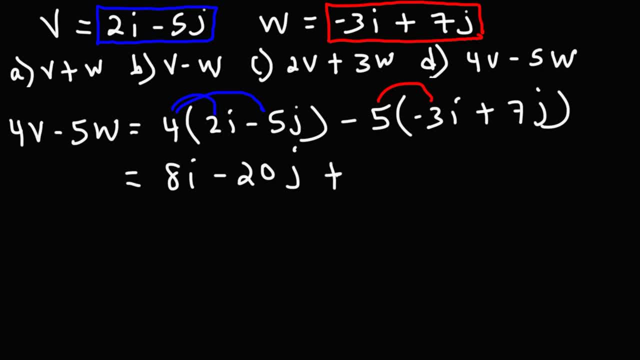 Next, we have negative 5 times negative 3i. That's going to be positive 15i. And then negative 5 times 7j. 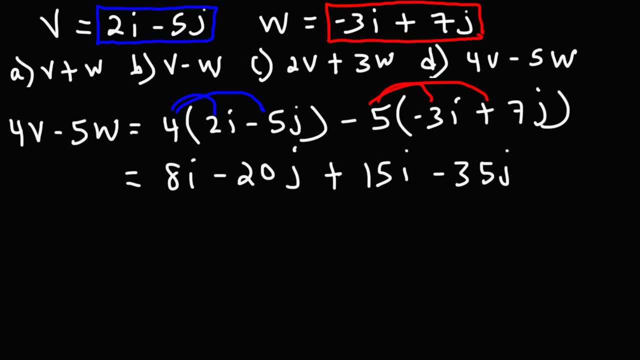 That's negative 35j. Is that right? It's good to take a minute to, like, check your work to make sure everything is done correctly. 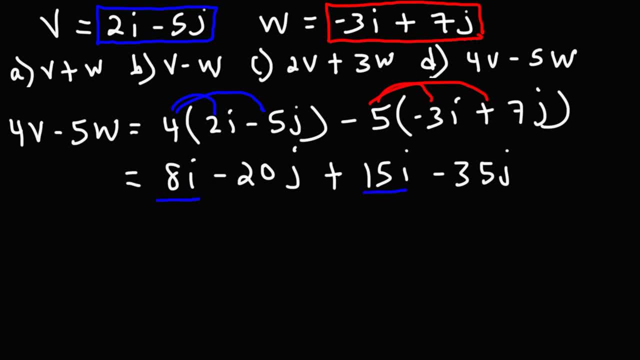 Now, let's combine like terms. 8i plus 15i is 23i. Negative 20j minus 35j. That's negative 55j. So that's it. 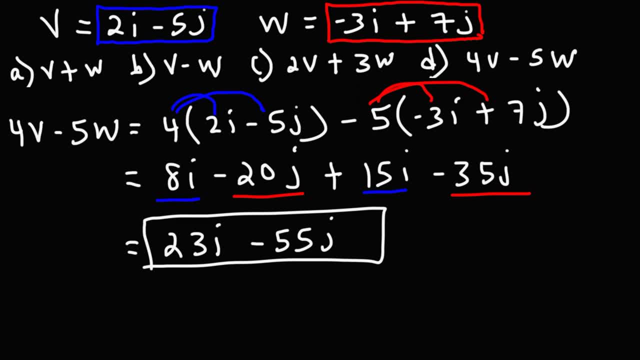 23i minus 55j. Negative 15j minus 35j. Negative 15j minus 35j. 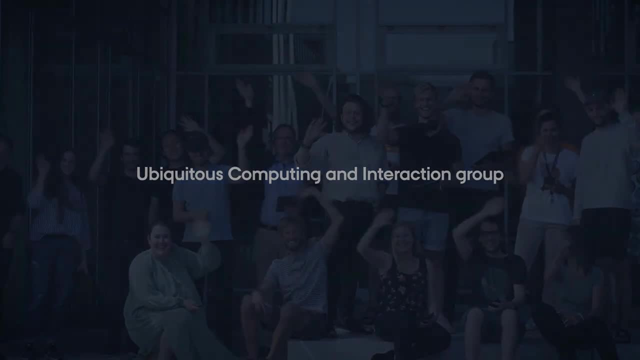 We live in a world where digital technologies are integrated in most aspects of our lives. We actively use smartphones, both at work and at home. We use smart watches for fitness and health, We use interactive office equipment for collaboration and many more things. My colleagues will give concrete examples on concepts and prototypes that we currently